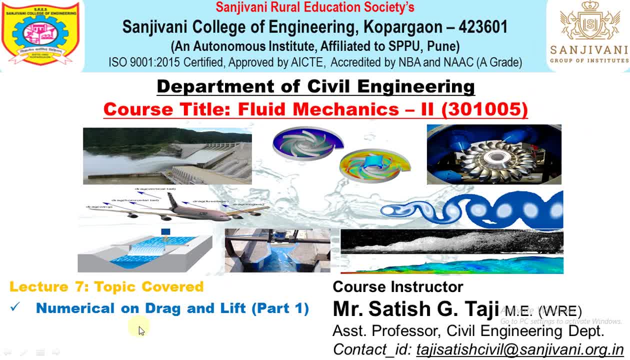 Hello everyone, this is our 7th lecture on the course titled Fluid Mechanics 2.. Up to the 6th lecture, we have discussed various topics like, say: concept of drag and lift, expression and derivation for the drag force and lift force, various types of drag, various types. 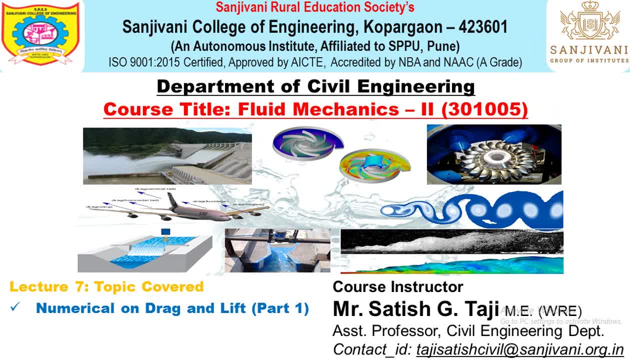 of bodies and factor effect which are going to affect the drag force which is acting on the body. And after discussion of all those things, we are going to solve some numericals In this lecture. we are going to solve some numericals. I have just splitted a lecture on the numerical into 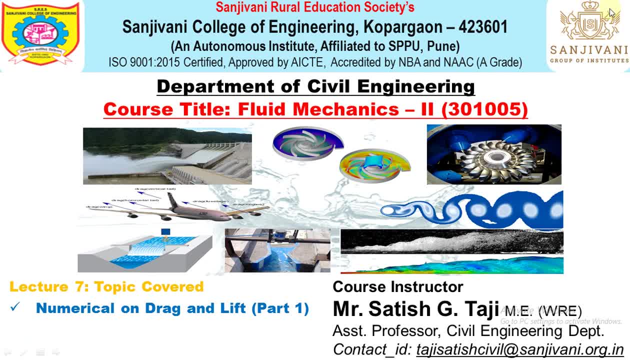 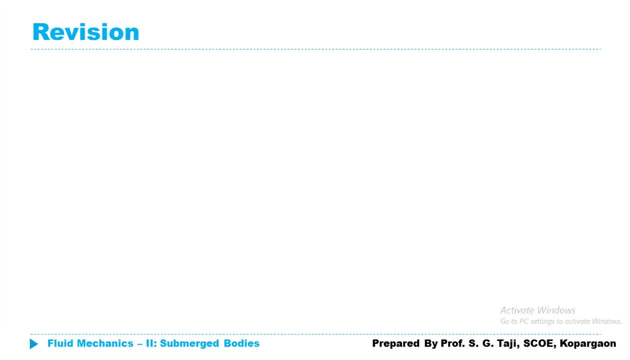 two parts. In the first lecture we are going to solve some simple numericals which are based on the equation of the drag force and lift force. As usual, before proceeding for this lecture, we will go through some previous topics, that is, we will make some revision. So drag force: 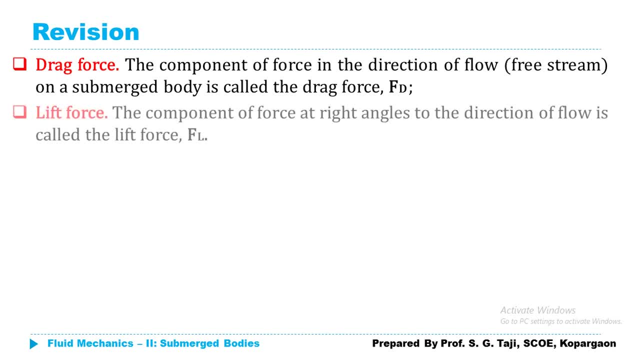 as we all know, it is a component of the total force which is acting in direction of motion. lift force: It is also a component of total force but it is acting in normal to the direction of motion. Again, expression for the drag and lift- as we have discussed drag force can be- is given by the 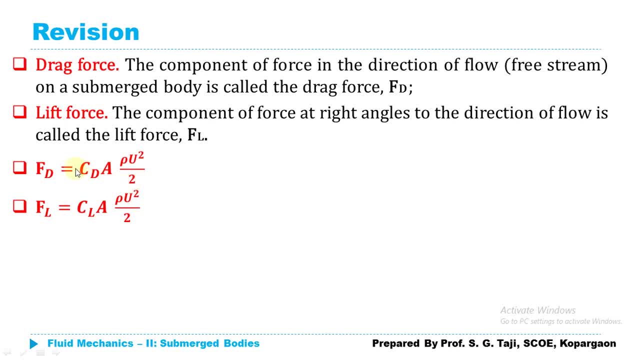 equation: CD multiplied by A, multiplied by rho, u square upon 2.. And again, lift force, which is given by coefficient of lift multiplied by A, multiplied by this dynamic pressure, rho? u square upon 2.. Just remember that rho and u are the density and velocity. CD and CL are the drag. 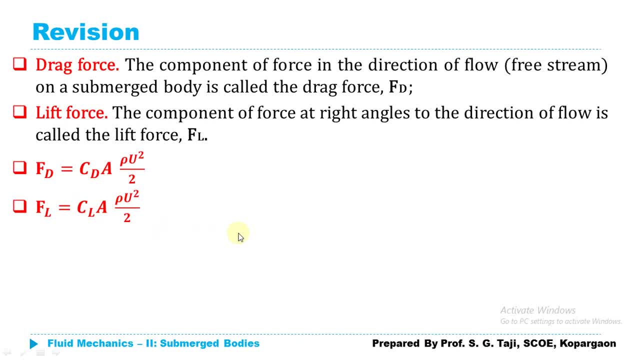 force and lift force, And this A which is going to play, is going to play a very important part while solving the numerical which is given by the which is known as projected area of the body in direction perpendicular to the motion or largest projected area of the submerged body. So, if you are considering submerged body, 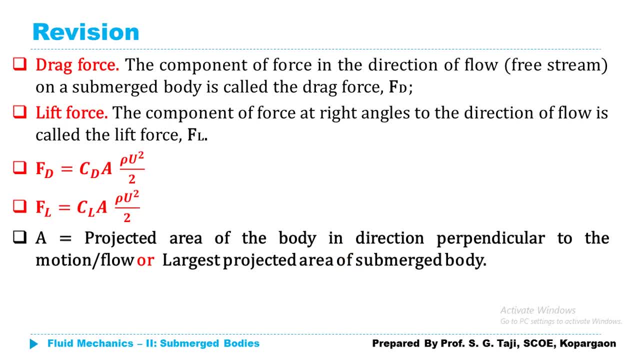 or anybody which is in air or in water, which is totally submerged, as we all know what is submerged body, which we have discussed in the very first lecture. So whenever we are considering submerged body, it is largest projected area of the submerged body or 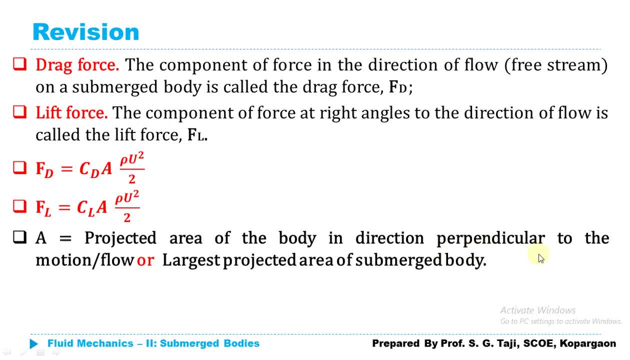 largest projected area of body in direction perpendicular to the motion. Now, whenever we are considering drag force, at that time we need external power to overcome the drag If we want to, you know, keep our object in motion. So at that time we need to overcome the drag and we need 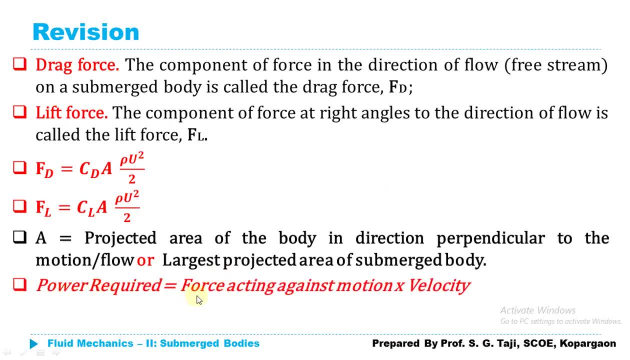 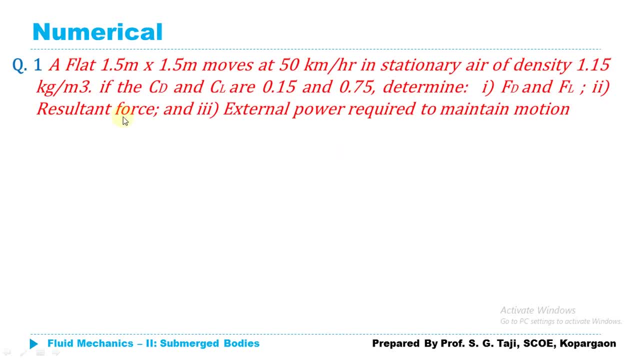 external power, and that external power can be calculated by using equation: force acting on that body against motion multiplied by velocity. So let's start this lecture with the numerical. a flat plate having area 1.5.. 1.5 meter by 1.5 meter moves at a speed of 50 kilometer per hour in the stationary air. 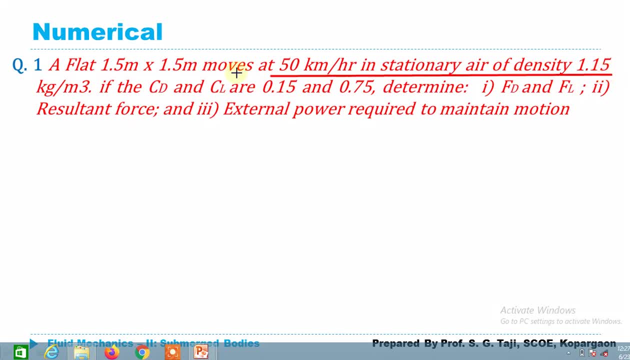 My plate is moving in the stationary air which is having density 1.15 kg per meter cube. If CD and CL- both are given as 0.15.75, then determine drag force and lift force on the plate or resultant force on the plate and external power required to maintain that motion. So 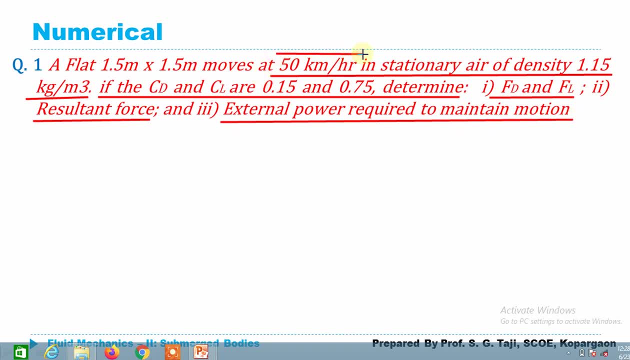 how much power we required to maintain the motion of plate as 50 kilometer per hour. So let's solve this numerical. Before starting, just write down all the given data. what they have given, Area of the plate is given as 1.5 multiplied by 1.5.. 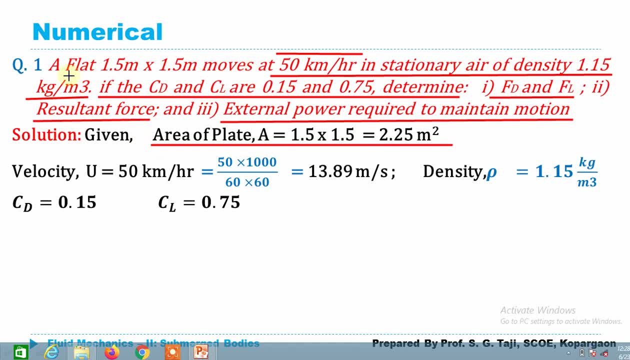 As we are considering air, stationary air. So if I am considering air, my flat plate will become a totally submerged body. So in that case, area of the body will become 1.5 multiplied by 1.5. So my area coming out as 2.25 meter. 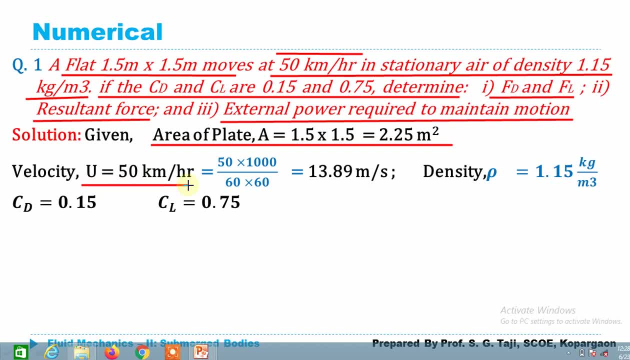 meter square. Again, velocity is given as 50 kilometer per hour. So I am just simply going to convert it into a meter per second, which is given by 50, multiplied by 1000, divided by 60, multiplied by 60.. 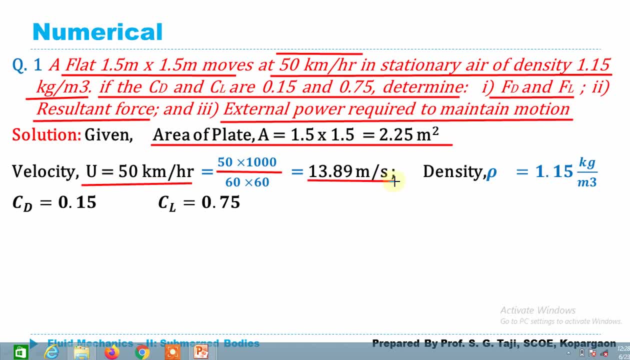 So my velocity coming out as 13.89 meter per second. Density of air is also given 1.15 kg per meter cube and we never going to convert that density. and CD and CL, both are given as 0.15 and 0.75.. So we are going to calculate drag force and lift force on the plate. So we are going to. 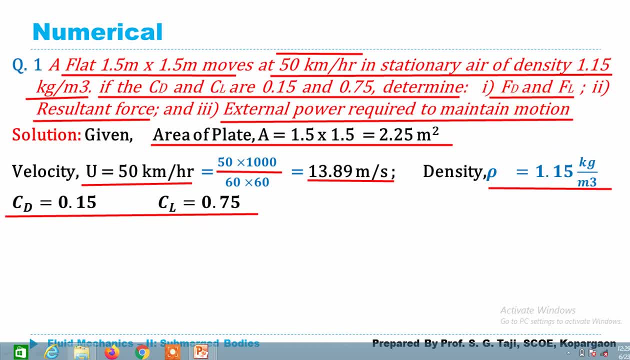 calculate drag force and lift force one by one. So first we will calculate drag force and lift force. As we all know expression for the drag and lift. So by using simply their equation we can compute drag force and lift force. Just put all the values respected value in those equations. you 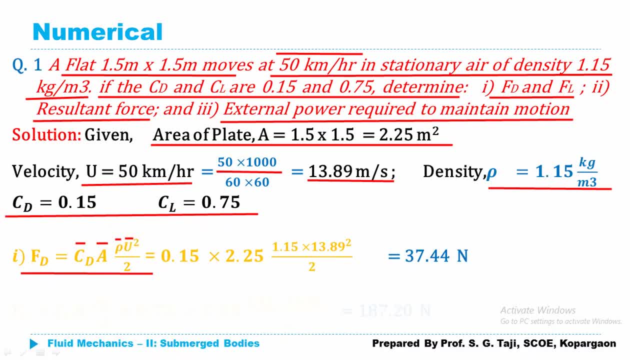 will get the value of drag force and lift force. So for the drag force, my value is coming out as 37.44 Newton and for the lift force, my value is coming out as 187.20 Newton. Just remember that the value of 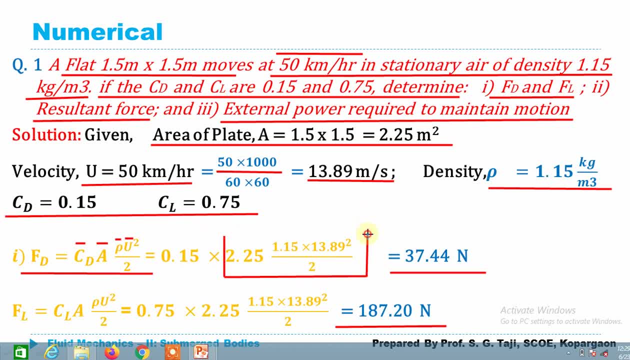 this part of the equation will remain same for the both drag force and lift force. Just simply it is going to change in drag coefficient and lift coefficient. So in case of drag coefficient it is given as 0.15 and for the lift it is given as 0.75.. So next we are going to calculate. 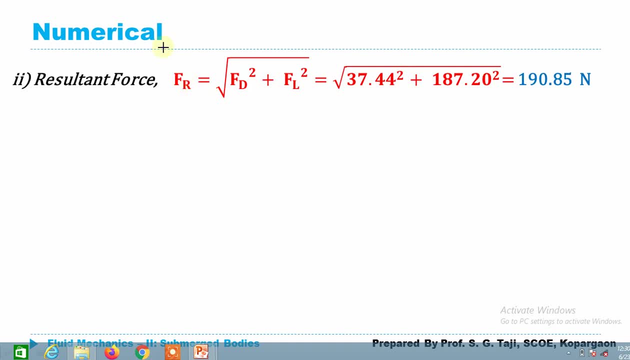 the resultant force, which is given by equation FR, is equal to under root of FD square plus FL square. So just put, simply put values of FD and FL, you will get the value of resultant forces: 190.85 Newton. Now I am going to calculate power required to overcome the drag, As we all know. 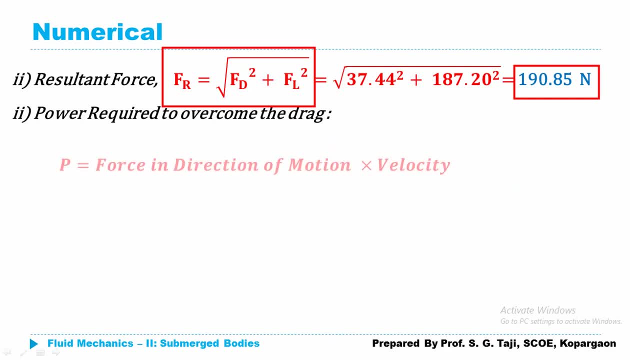 power required to overcome drag will be given by the equation: Power is equal to force in direction of motion multiplied by velocity. Now, which force which is going to act in direction of motion? that will be only a drag force and it is going to act in direction of motion. So I am just simply going to put that. 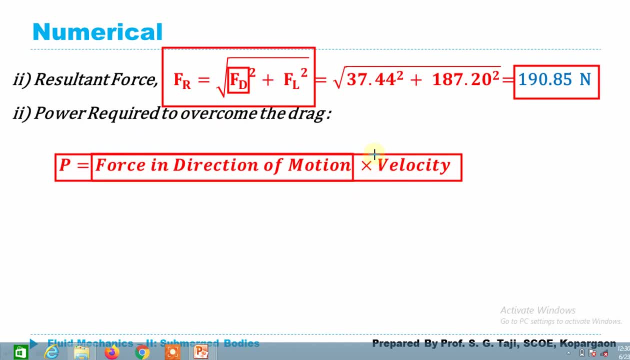 value of drag force here and velocity. So I need to maintain velocity of the plate as 13.89 meter per second, So I am going to use that value here. and how much power I required to overcome the drag. that will be coming out as 519 watt or 0.519 kilowatt. So this is our solution of this. 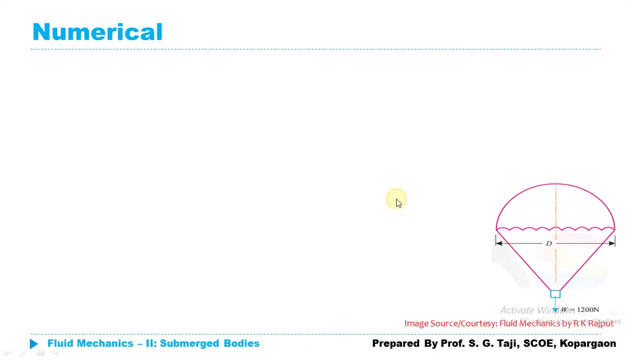 particular numerical. We will move to the next numerical. So this is our solution of this particular numerical: We will move to the next numerical. We will move to the next numerical. So this is our solution of this particular numerical. We will move to the. 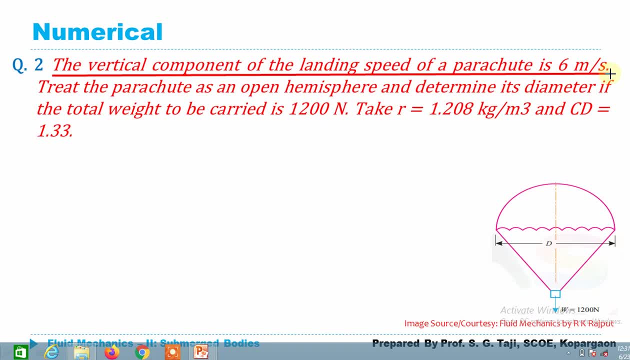 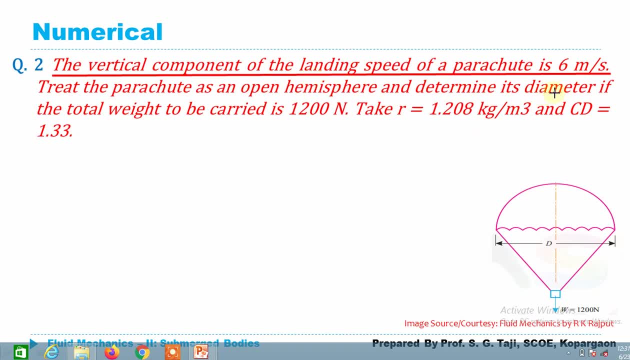 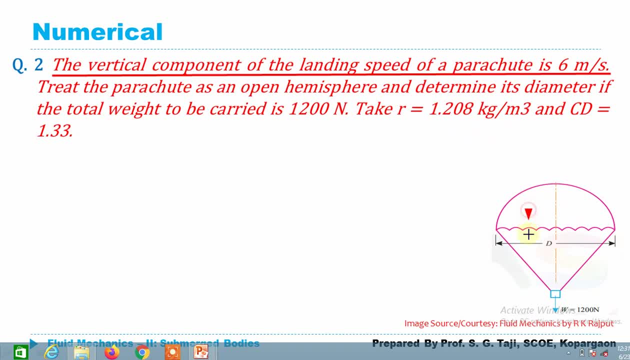 numerical. So this is our solution of this particular numerical. So this is our solution of this particular direction, but its vertical component of that velocity which is acting in downward direction, and that velocity component is 6 meter per second. that is mean that it is coming in downward direction with the velocity 6 meter per 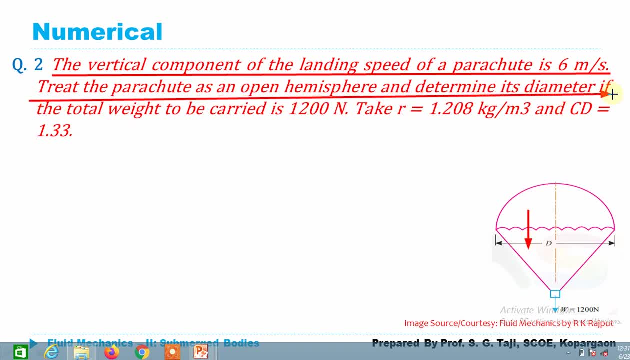 second, treat parachute as an open hemisphere and determine diameter if the total weight is to be carried by the parachute as 1200 Newton take. value of R is equal to sorry. sorry, here it is not R, it is given as 1.208 kg per meter cube. 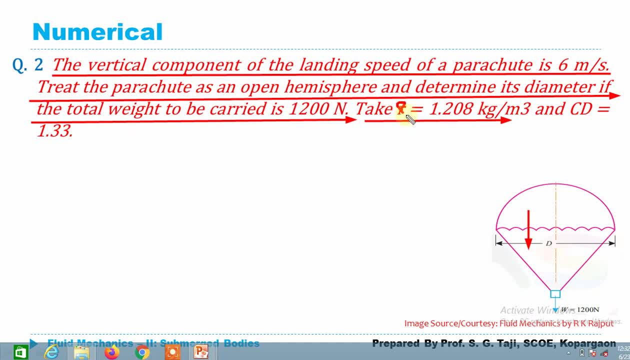 that is mean that it is density. mistakenly I have taken there are, so I'm just going to replace it with the density. I'm just going to correct it. and CD is given as 1.33, simply the arts to calculate diameter. diameter, that hemisphere, that parachute, and we're going to treat that hemisphere as a that. 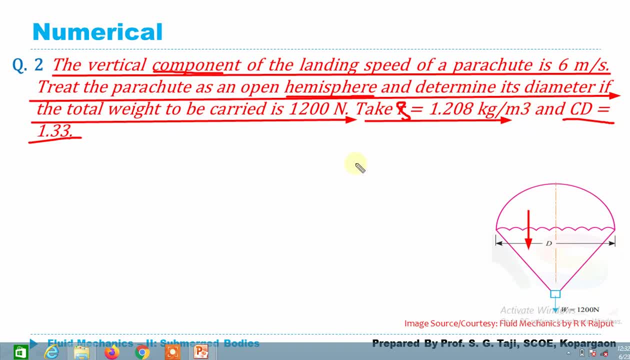 parachute as a hemisphere, we need to calculate its diameter. so whenever we are considering that parachute as a hemisphere, in that case area of that hemisphere will be given by pi by 4 multiplied by d square. so i am just simply going to use this equation and i am just going to replace that this equation. 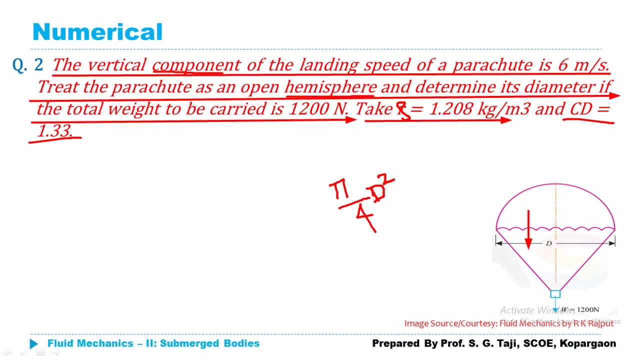 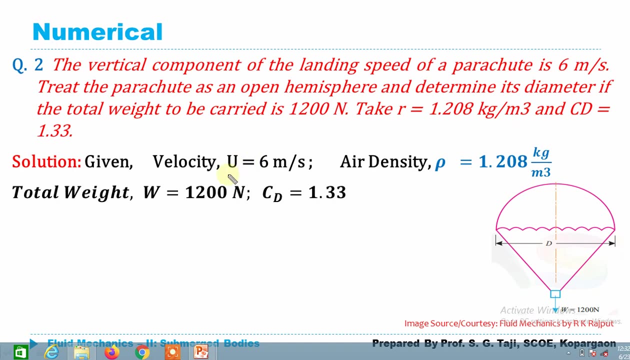 this value of the area in the drag equation. so i will get the, this value of the diameter. so let's start, before proceeding solving to the numerical, we will just write down all the given data. so what they have given, they have given velocity: a 6 meter per second. 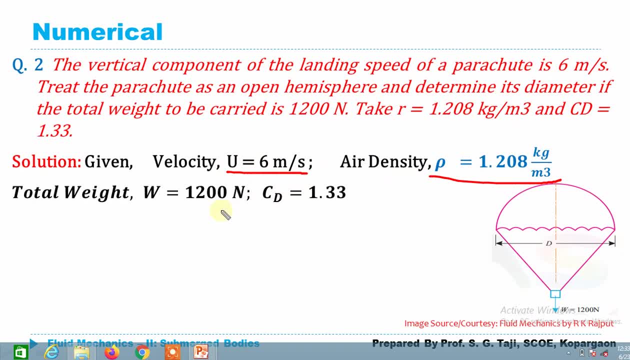 downward velocity. they are also given air density as 1.208 kg per meter cube. they also given the weight which is carried by the this parachute, that is mean that it is going to act in downward direction that weight component and cd that is given as 1.33. as i am treating my hemisphere, 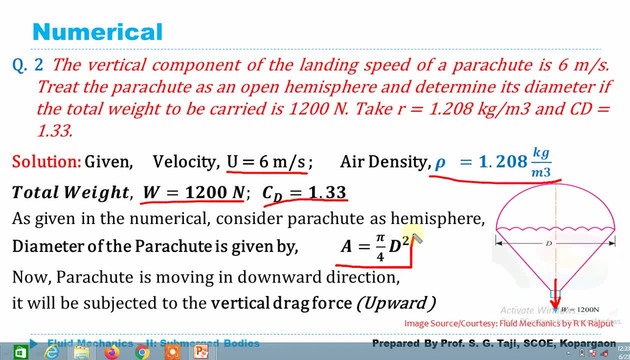 parachute as a hemisphere. in that case, uh value of the area will be given by pi by 4 d square. now, whenever my parachute, which is coming in downward direction, as it is coming, moving in downward direction through air, at that time it will be subjected to the drag force which is acting in upward direction now, both force acting. 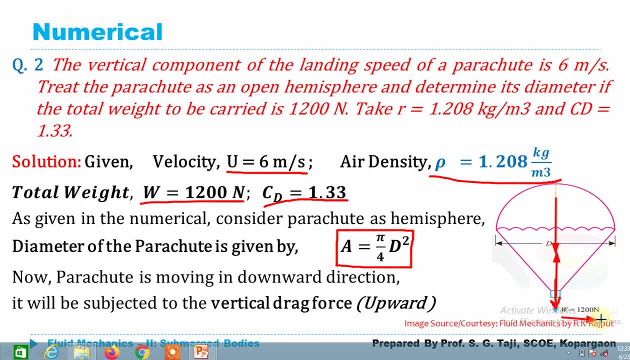 in opposite direction. now downward component. we know weight component, which is given as 1200 newton. so with the weight of 1200 newton, my parachute moving in the downward direction, at the same time it will be subjected to the drag force. now if i, if i want to maintain my 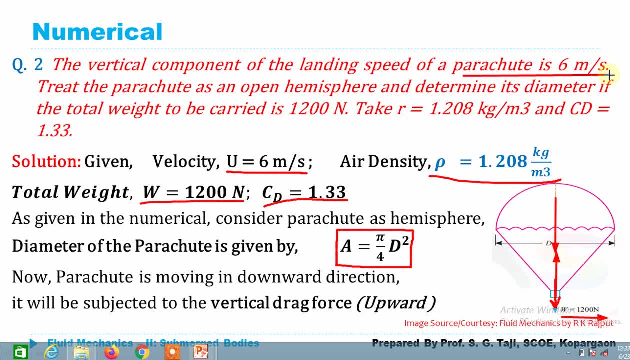 speed of the parachute as 6 meter per second. in that case, whatever my drag, which is acting in upward direction, and weight component, which is acting in downward direction, both should be equal. if it is not equal, like say if my drag is greater than weight, whatever the weight component. 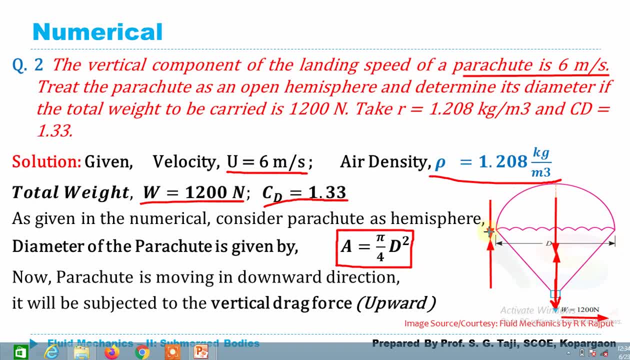 and drag component. if my drag is greater than this weight component, in that case my this parachute will be lifted in upward direction. it won't come in downward, uh, never going to land on the ground. so if my this drag, which is acting on vertical direction, is less than the weight, it that in that 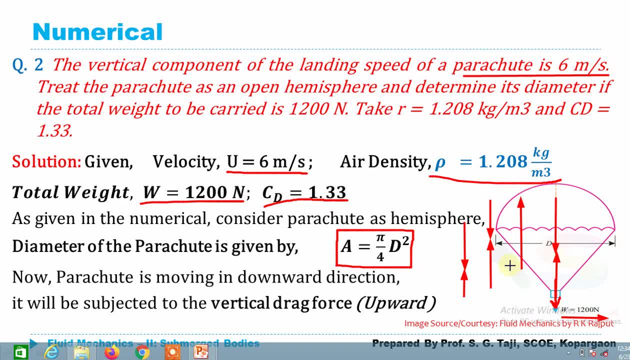 case, whatever the speed of my parachute is going to increase in the downward direction, so it will become faster, it will reach faster on the ground surface. so to maintain that velocity, i need to uh, we need to uh maintain our drag and weight component as equal. so i am just simply going to 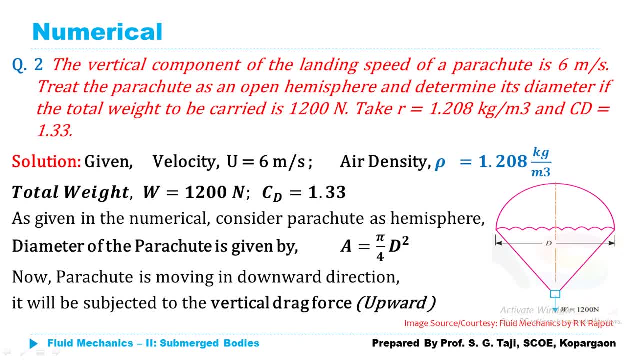 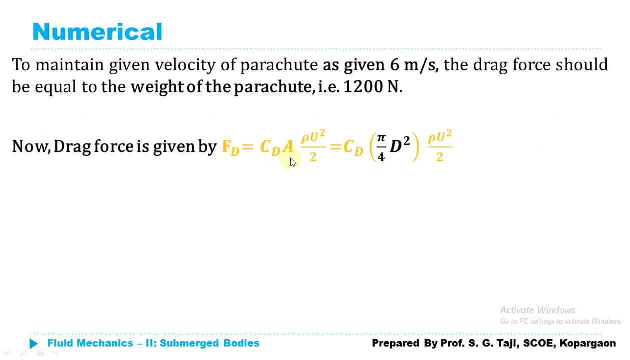 use my value of drag in the equation of drag as 1200 newton per second, which is equal to the weight, and i am simply going to calculate the diameter. so we know that uh, equation for the drag which is given by cd, multiplied by a, multiplied by rho, u square upon 2. just replace this a with the pi by. 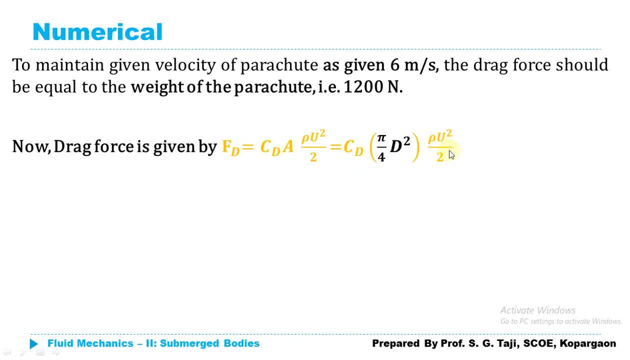 4 d square and cd is already given, rho u square upon 2, velocity is already given, density is already given and for that velocity we know that we are just going to equate my weight and drag and just i am going to replace the drag with the 1200 and by putting all the respected values 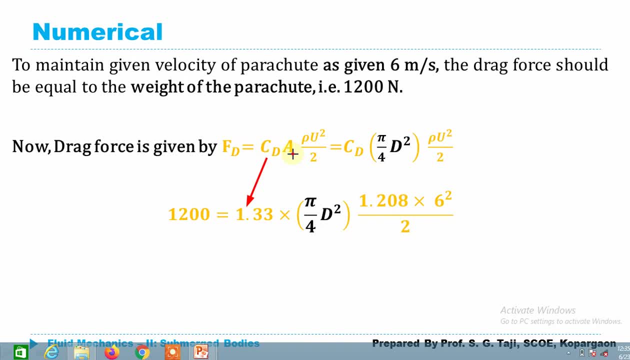 by putting all the respected value as cd, as 1.33 area is pi by 4 d square. we are simply going to calculate d. here again, density of air is given as 1.208, velocity is given as 6 and fd, which we have taken equal to the weight component, and after considering all, 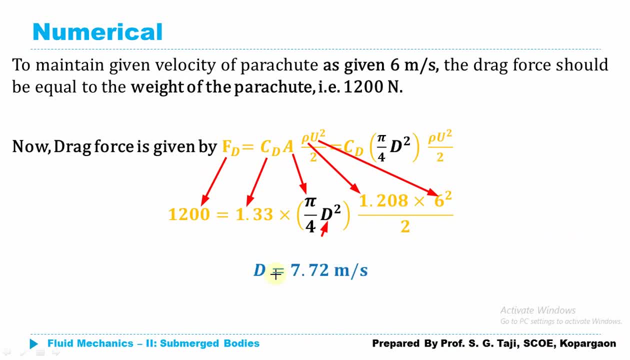 those values and after doing the calculation, i am getting the value of d as 7.72. sorry, it's not a meter per second. again, i have just typed there meter per second, so it is 7.72 meter. so this is our answer. those are the simple numerical based on equation of the drag force and lift force. 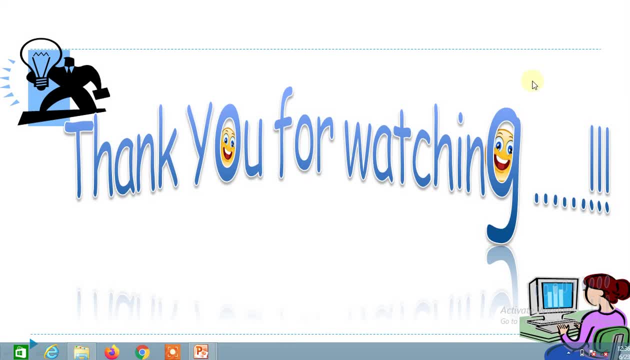 in the second, next numerical, where we will solve some other and some tricky numericals. so that's it in this lecture. thank you for watching.